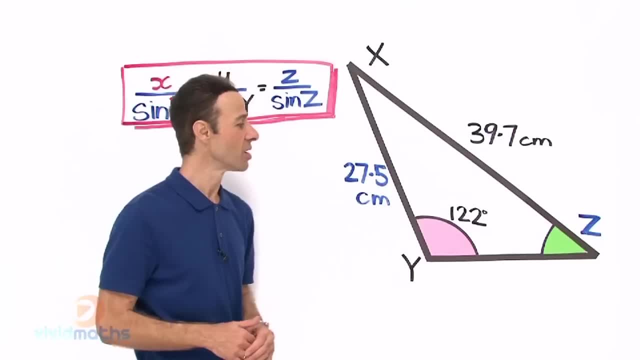 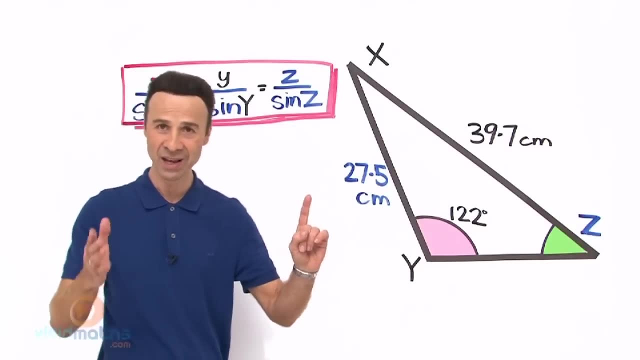 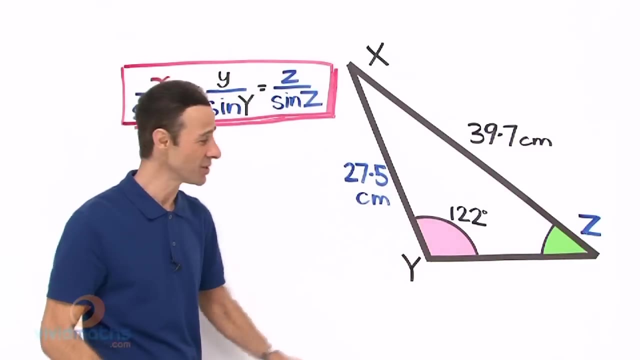 angles and the little letters refer to the lengths. so, what do we have here? we have this triangle here and we are given three pieces of information. we are looking for the one missing one, as I said, the missing angle right down here. Now, what do we have? well, we have another angle here. it is 122 degrees, it is angle Y and opposite. 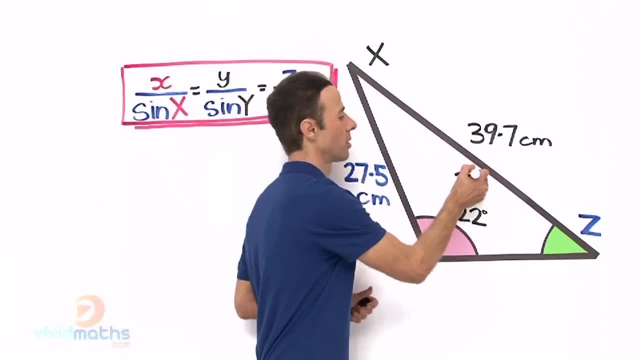 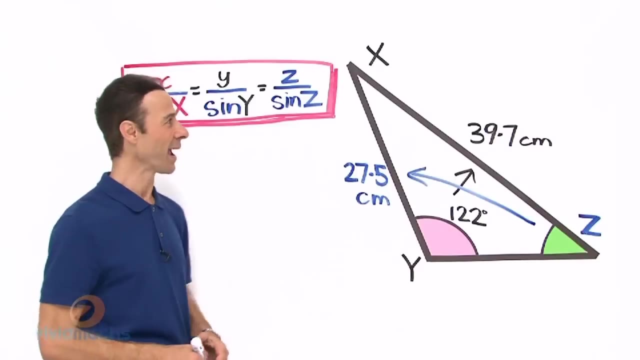 directly opposite, that is, the length 39.7.. Now, the angle Z that we are looking for is directly opposite the length 27.5. we are going to take these pieces of information and install them into this formula up here, the sign rule, which you have done before, so let us put them. 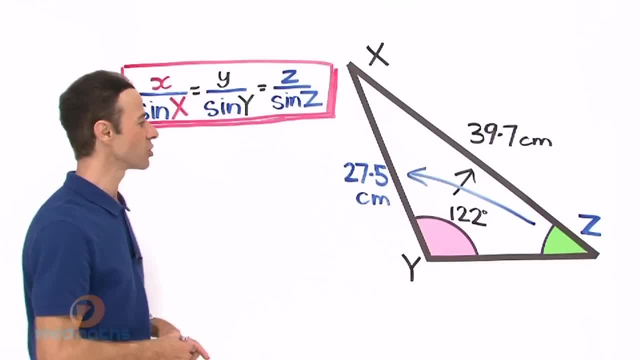 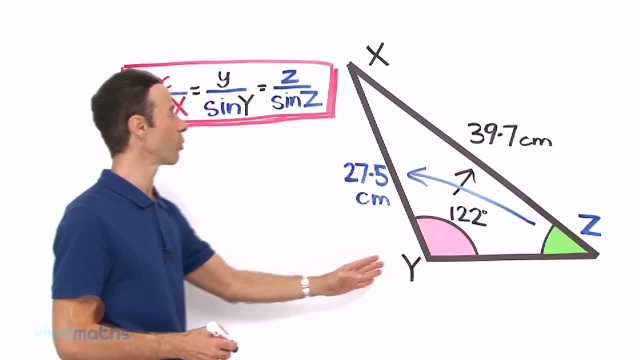 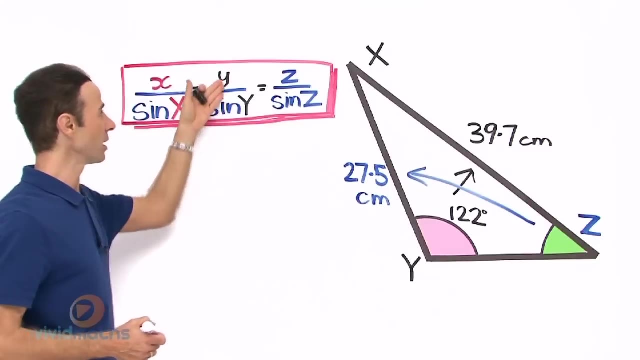 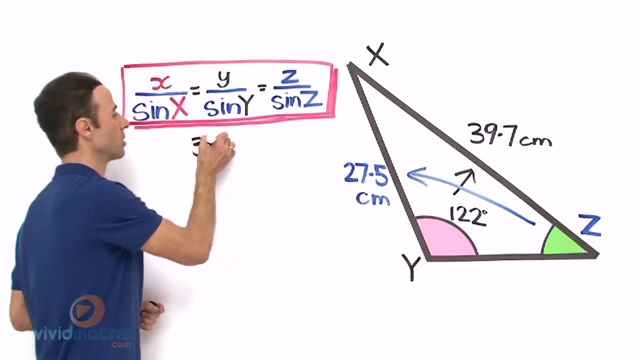 in there. so, taking a look at what we have, we have straight away- we have 39.7cm opposite the Y. so let us start off with the Y. it is Y little Y over sign Y capital. the Y is the angle, so let us put them in here. so little Y, 39.7, let us put that in there. so that is. 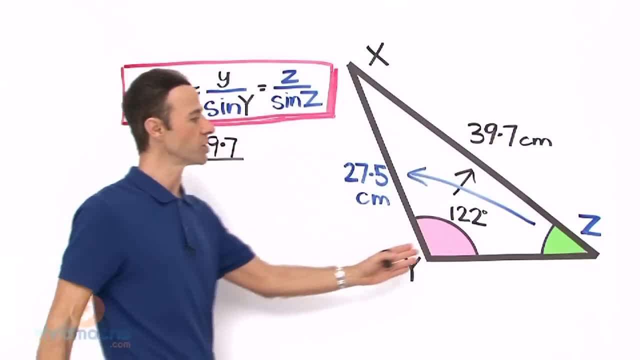 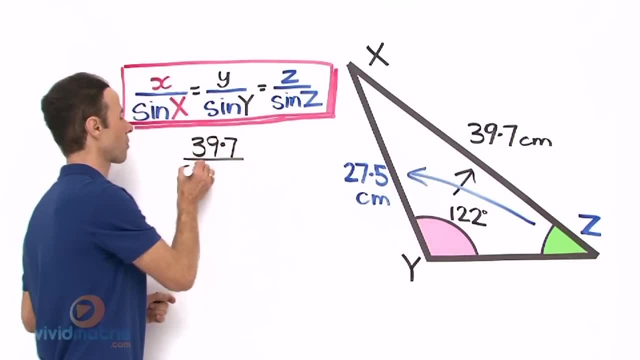 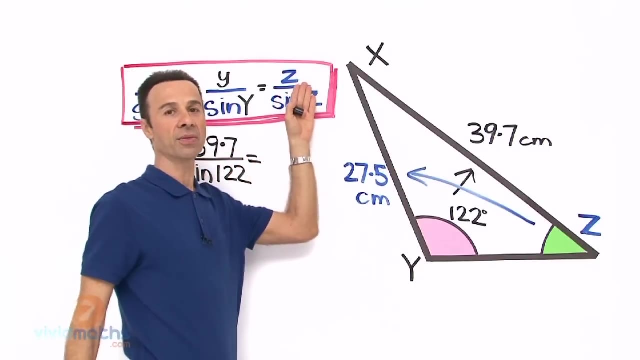 39.7. all over sign Y, which is the angle down here, directly opposite. can you see that? yeah, 122 degrees. Now that is going to equal Z. right, that is the distance, Z, which is right here, 27.5, let us put that in there. all over the angle directly in front, the missing angle. 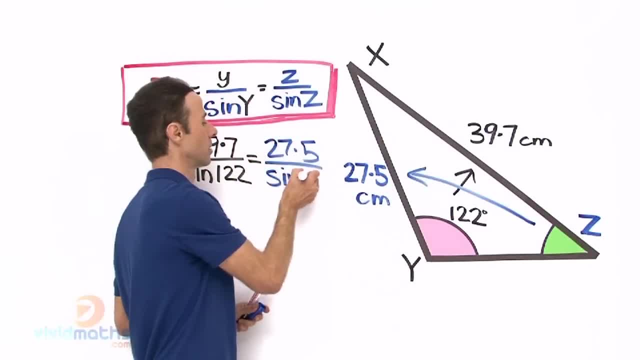 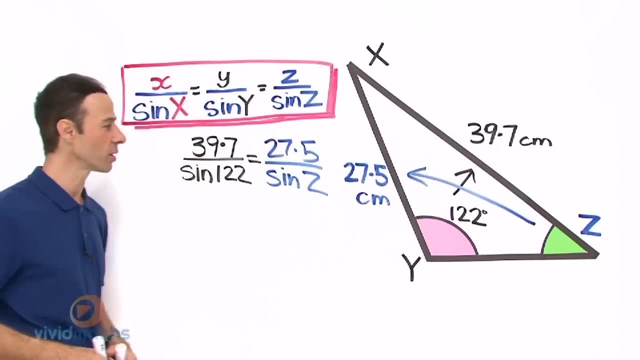 sign Z. Ok, there is our pieces of information: 3 unknown. 1 unknown. the angle up there is what we are looking for. so what do we do? as always, we cross multiply. so let us do that, let us cross the multiply all the way across, so we will have. 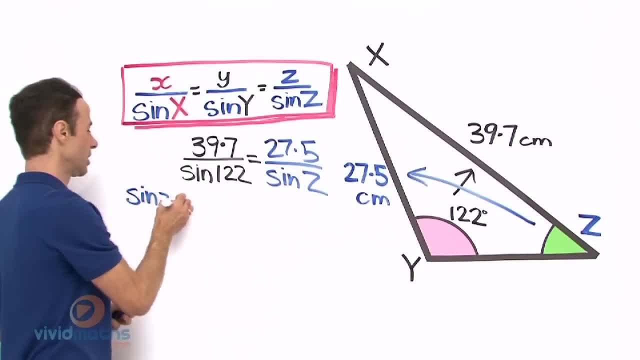 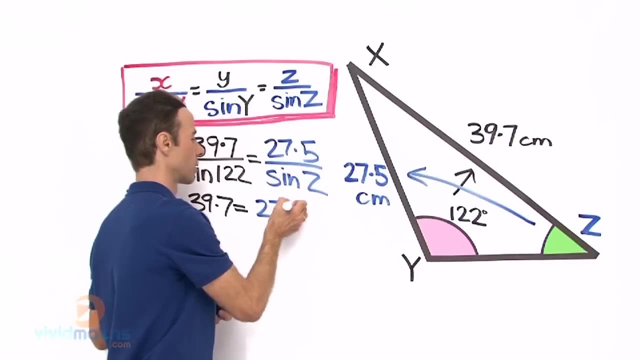 Sine Z times 39.7 equals. that is going to be 27.5 times sine 122.. Ok, what do we want to get to? Sine Z times 39.7 equals that is going to be 27.5 times sine 122.. Ok, what do we want? 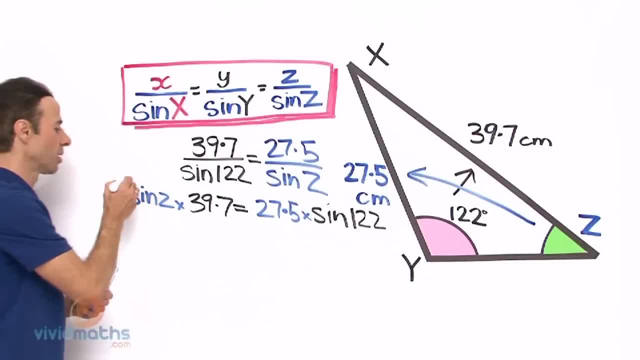 to get to Sine Z times 39.7, equals that is going to be 27.5 times sine 122.. Ok, what do we want to get to? Sine Z times 39.7, equals that is going to be 27.5 times sine 122.. Ok, we are going to. 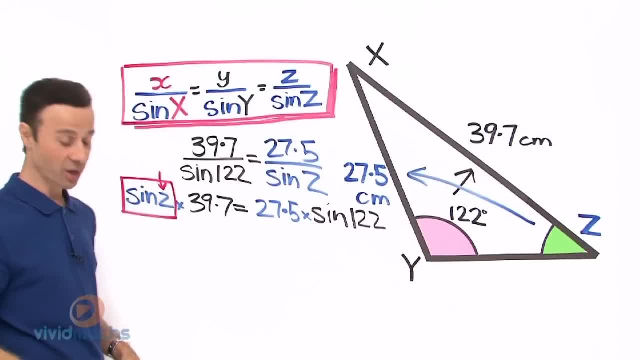 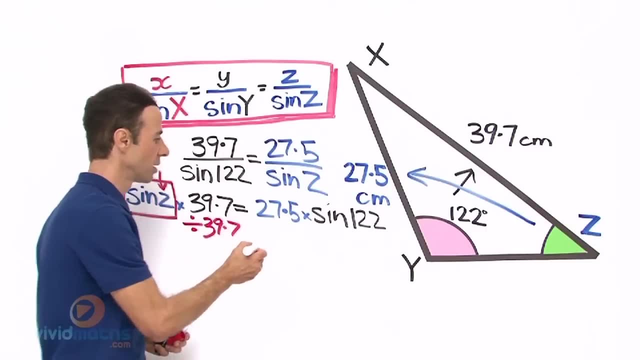 get to The constant, The constant. So this is a person that has 29.7 plus sine. we are going to get itlay 32, so that is going to get us to, As you can see, with three numbers. этот number eight, which is our, 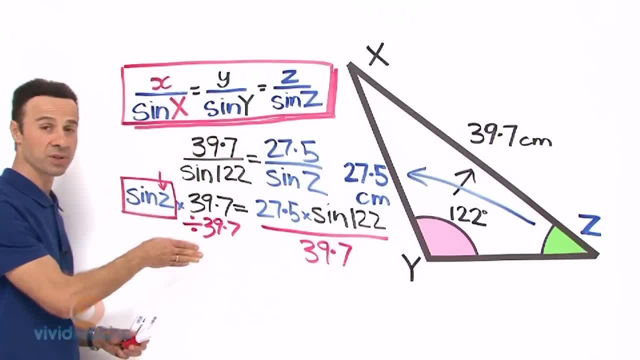 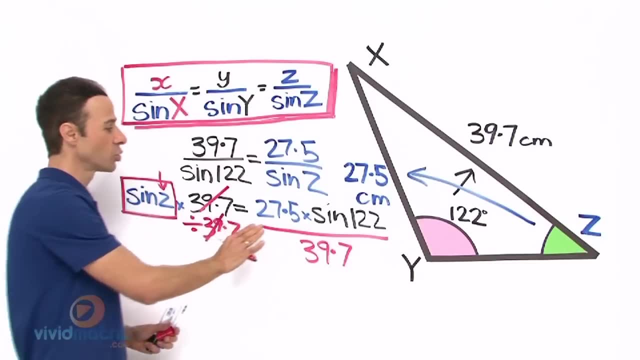 That is right here, the z, the little z here. that is the promo numero particular right there. that is what we are looking for. so let us divide both sides by 39.7, so let us do equals 27.5 times sine 122 over 39.7. let us put this stuff in the calculator right now. 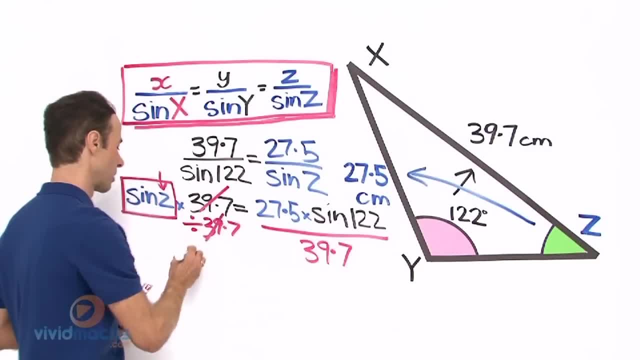 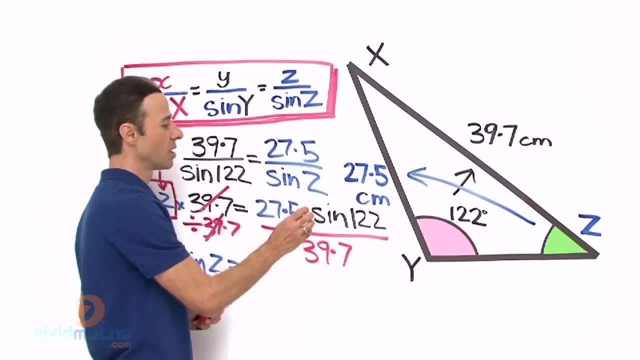 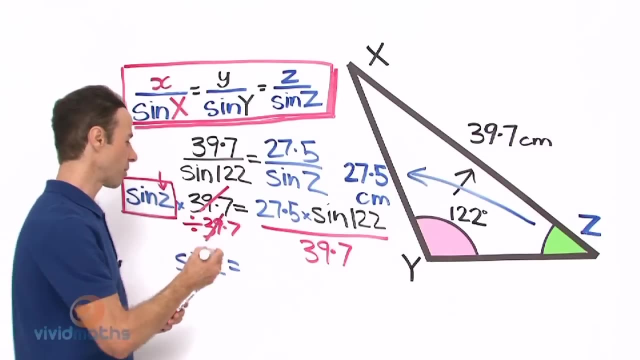 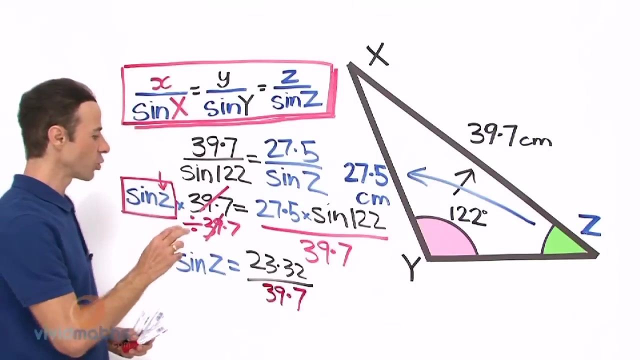 so we are going to get now on the calculator: 27.5 times sine 122. that is going to yield 23, that is going to be 23.32 all over what we have there, which is the 39.7. ok, let us put that in the calculator again: 23.32 divided by 39.7 is going to give us and equal 0.3. 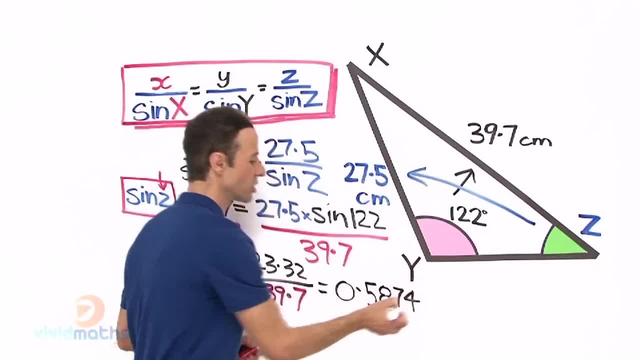 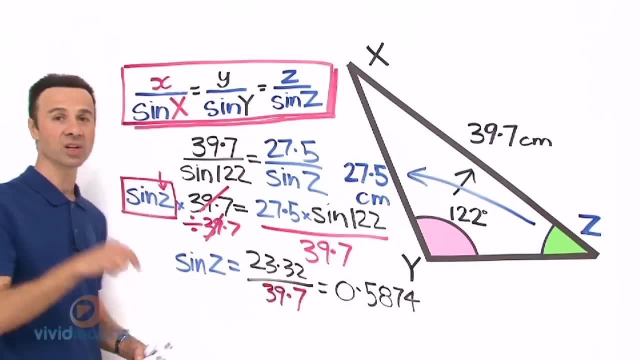 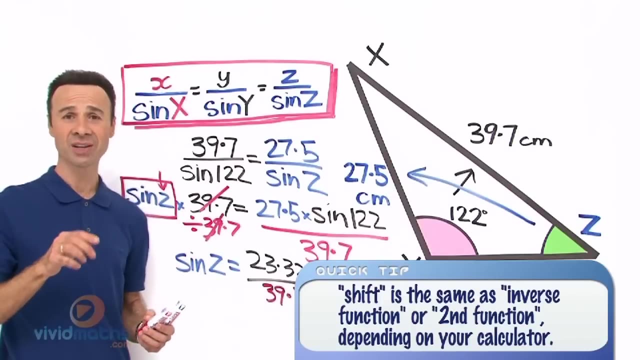 5, 8, 7, 4. we will just take it to 4 decimal places and then we are going to find z. now, to find z right here, sine z, we are going to shift z on that. so if you are on your calculator, depending on what you have, shift z, sine z, or second function or inverse, whatever you. 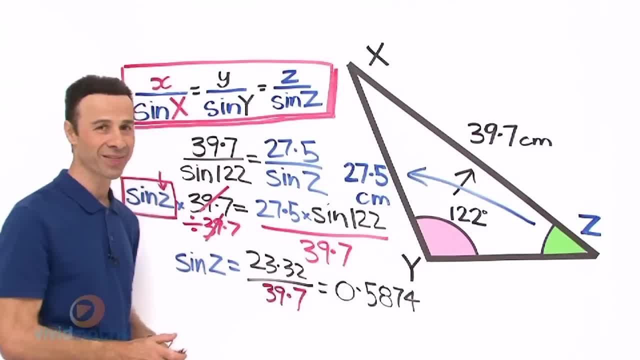 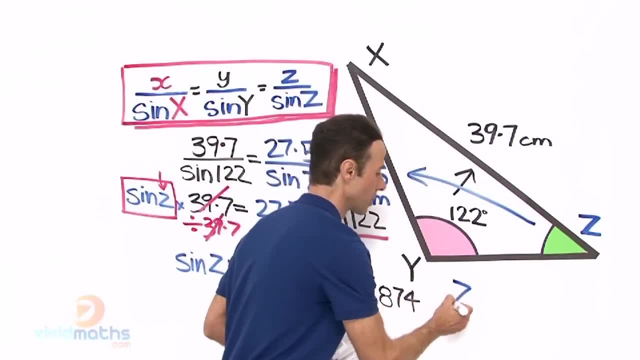 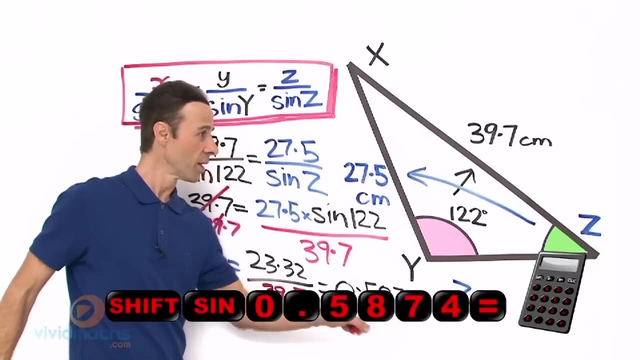 have on your calculator. so we are looking for z. what have we got? the angle right. here is what we are looking for. So capital Z, which is the angle. Ok, Equals. so you got shift sine 0.5874. that is going to give us to the nearest degree.